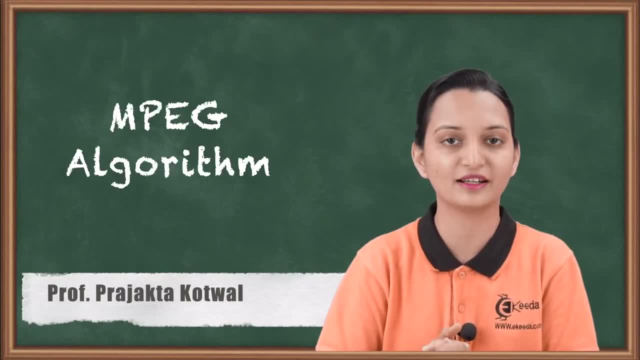 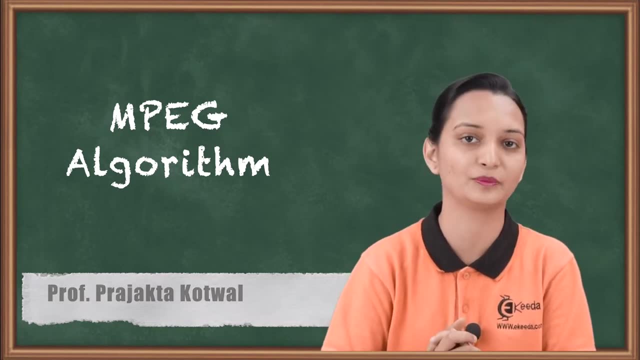 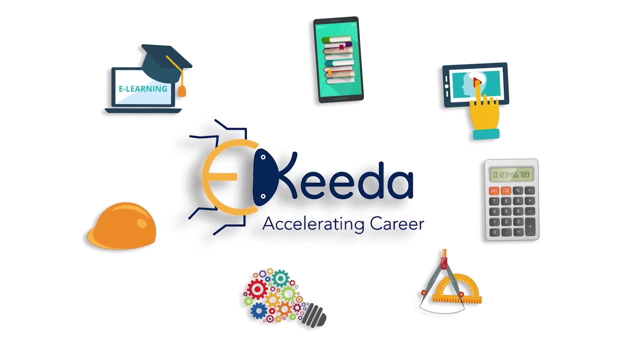 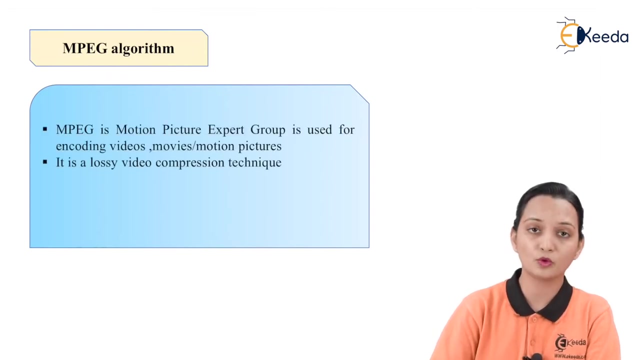 Hello friends, in this video we will try to understand the basics of MPEG algorithm after studying the compression technique along with the JPEG algorithm. So basically what it means by MPEG algorithm. MPEG is a motion picture expert group. MPEG is used for encoding the videos, movies or motion pictures. 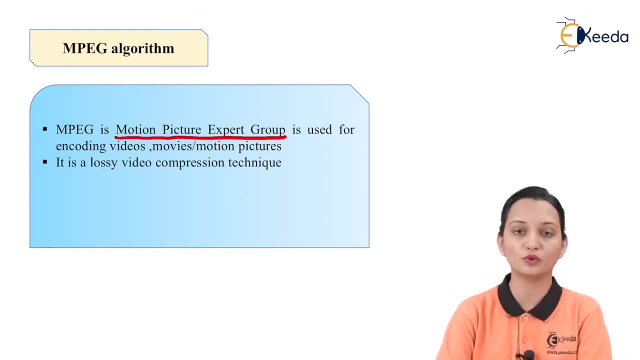 Now we are able to use JPEG also for the image compression purpose, Then why we are moving for the MPEG? The simple answer is to overcome the drawback which we get from the JPEG, And it can be possible by using the MPEG. But the most probably we go for MPEG only because of one more thing. 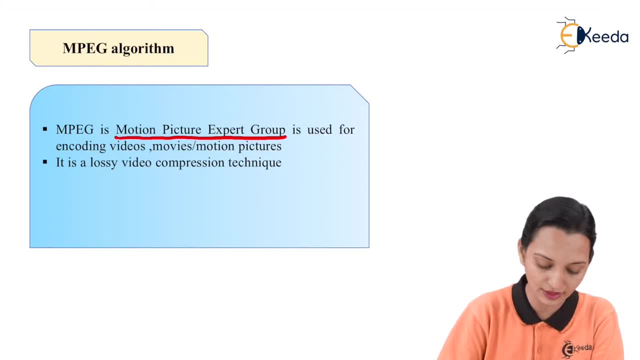 That is nothing, but it is used for the encoding videos, movies and specially the motion pictures. What it means by the video or the motion picture. JPEG is a technique which we can use for the image compression. This we have already studied And its algorithm is also very simple, which we can apply on the different parts of the image. 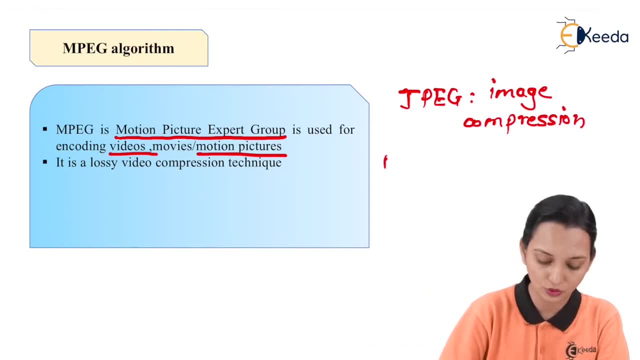 To get a better result. But though we are having JPEG in our hand, We move for MPEG only because MPEG will do. the encoding of video Means what Sequence of images at one time. That means a video is nothing but what. A motion picture is nothing but what. 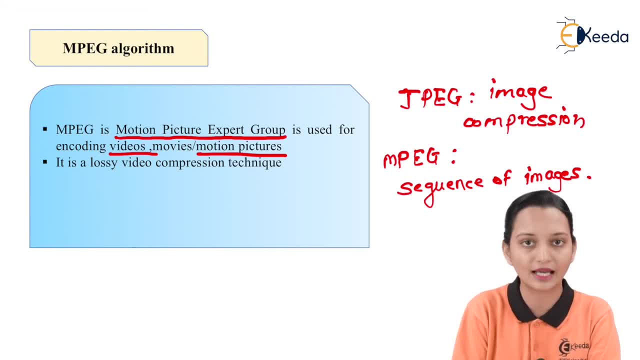 Sequence of images Which can be stable can be unstable. That means the image can be taken with the help of a single place, Or it can be taken with the help of the different places. So the sequence of images under encoding is nothing but what. 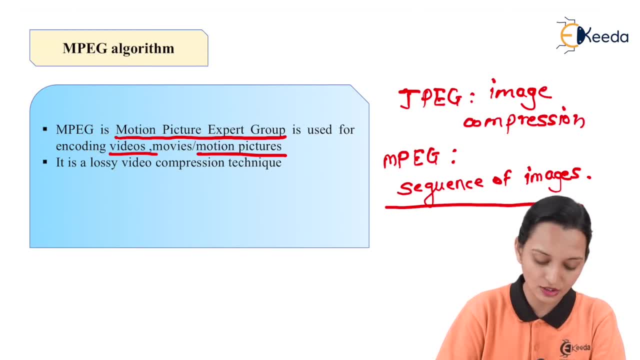 Use of MPEG. Now, MPEG is a lossy video compression. We all are familiar with the lossless and the lossy type of the compression technique. Lossy means what There will be, some loss of data, Actual- And this kind of data is nothing but the actual loss. 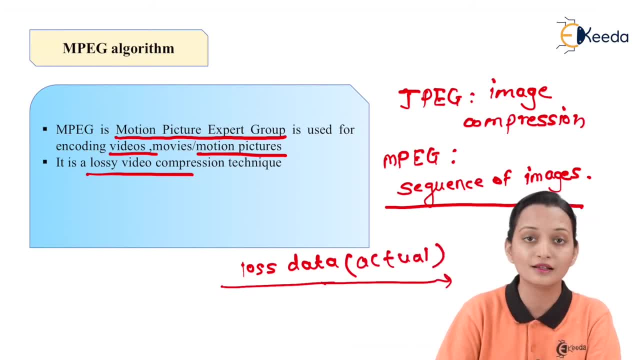 Actual data. The meaning of compression is compressed of size. That means decrement in the size. But the meaning of lossy technique is nothing but the actual loss of data. That means this is the sender and this is our receiver And in between that, if X is your number of message which you have to send towards your receiver, 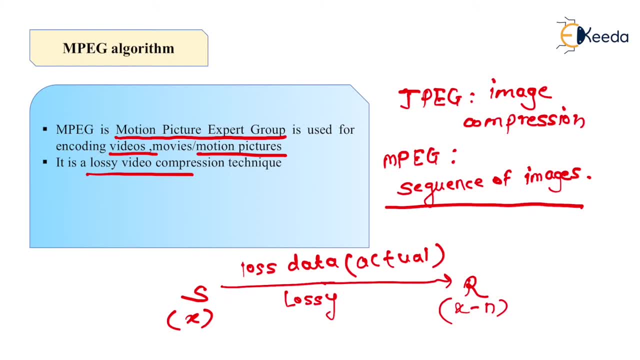 Actual loss of the data will occur in the lossy technique, And hence here you are getting what X minus N Such amount of data. So exactly what happen when you are going to use the lossy video compression: There will be the possibility of reduction in the actual data. 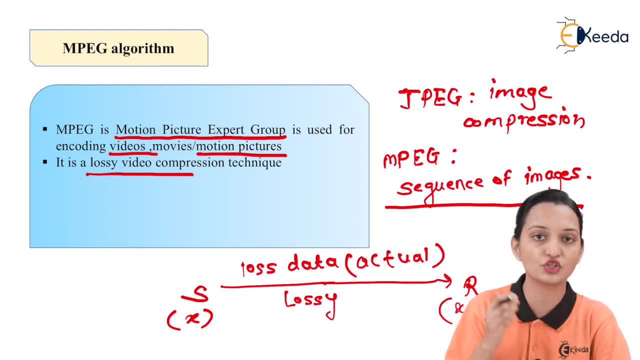 And which is not suitable for the compression or which is not suitable for the receiver side also. That we all know, But still we are going to use MPEG. That means here the actual loss of the data occur, But that data may not be useful or it may be the unwanted. 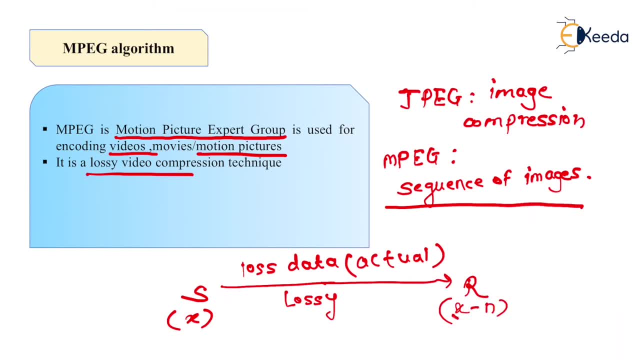 So maximum time it will loss the data. But this particular data- we can say this- can be the unwanted data. So what it means by unwanted data, then We all are familiar with a photo. That means a simple click with the help of a camera is nothing but a picture. 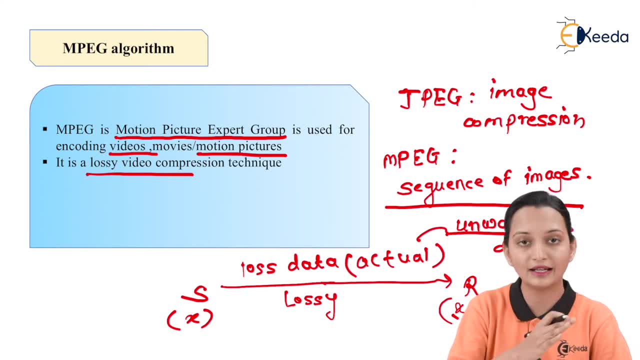 So in that picture we have to focus on a particular part And a part of that particular part. though the background is blur or though the background is light in a brightness, Then also it doesn't matters when we required to focus on a particular part of the image. 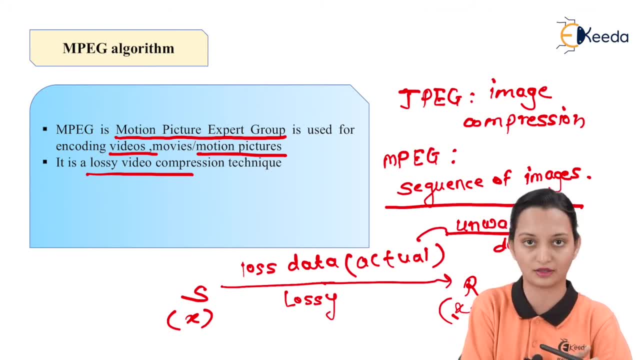 So such kind of unwanted part instead of that focused part Which we can do some coding or encoding on that part And which we can ignore, That particular data can be known as the unwanted data And that data can leads to the lossy compression with the help of MPEG. 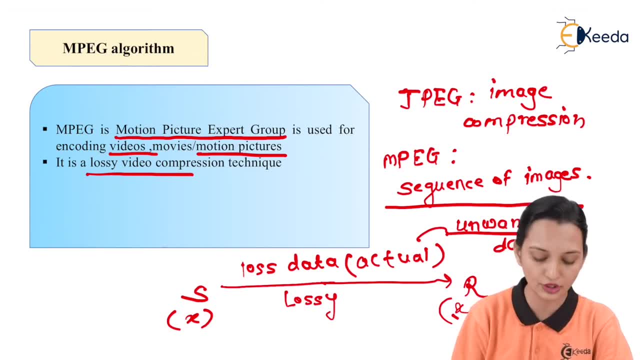 So, though the MPEG is nothing but the lossy video compression technique, Then also we are getting the maximum good results with the help of the MPEG. Why? Because that will loss the actual data, But that data may be the unwanted data. The next part is. MPEG requires continuous sequence of images to develop a video. 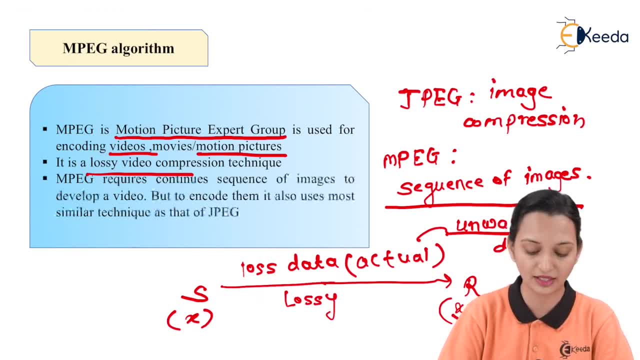 As we have already discussed, This is the difference between the JPEG and MPEG. Joint Photographic Expert Group is nothing but JPEG, Which will take one by one image, Means it will try to encode the first image, Then that will be the output number one. 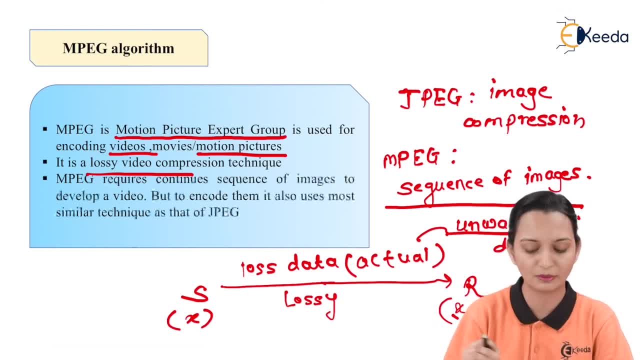 After that it will try to encode the second image, Which may be known as the output number two, like that, But in the MPEG input itself is nothing but the sequence of the images, So that the video can develop. So development of a video is nothing but the sequence. 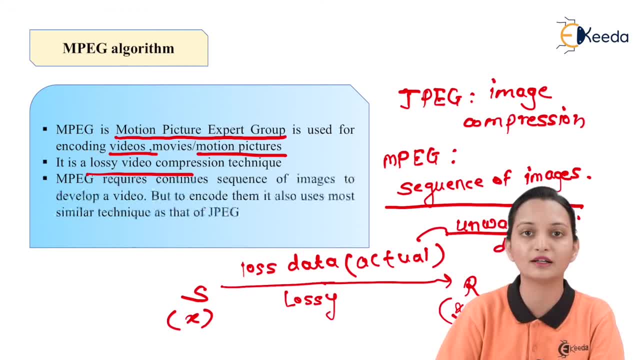 The sequence of images and its encoding can be done with the help of the MPEG, Which is known as Motion Picture Expert Group, But to encode them it also uses the most similar technique as that of JPEG. Then why it can use the most similar technique, like JPEG? 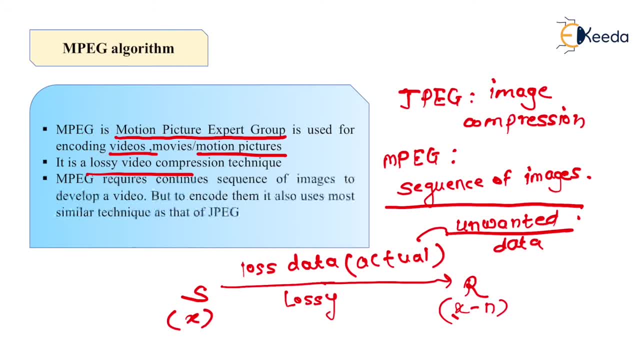 Because in the JPEG also there will be the compression of what Compression of image that can be takes place, And in the MPEG also there is a compression of what Compression of sequence of images. So the basic component of which we have to take the compression is same. 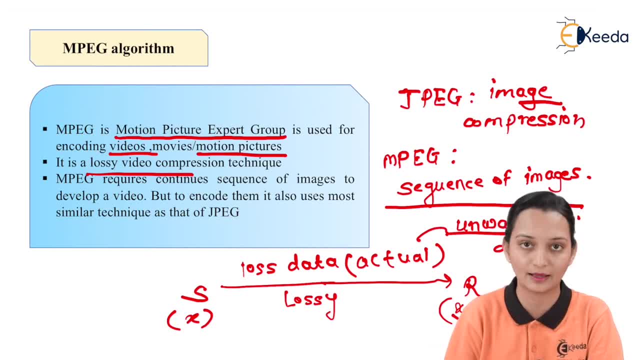 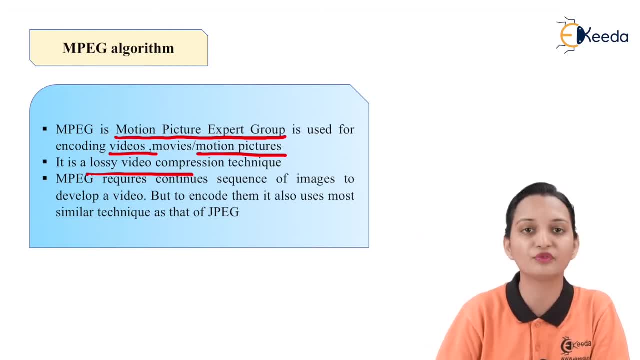 So that the encoding technique is also same or much more similar as that of JPEG for MPEG. Now exactly what it means by MPEG file storing, Because after the compression with the help of MPEG technique, we have to store the file Like after the compression of JPEG. we can store the file like a JPG. 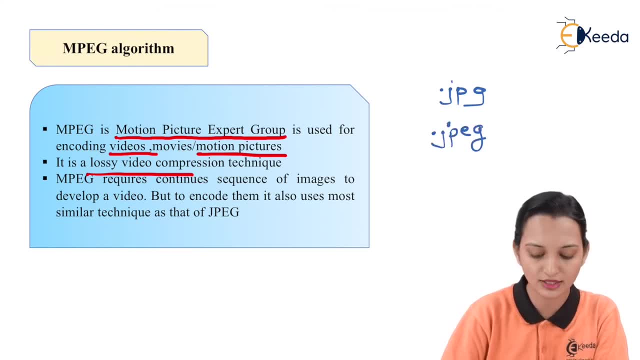 Or like JPEG. So this is nothing but what Compression format of a file with the help of the JPEG technique, Now with the help of MPEG, how to store the file? mp3, mp4 And hope. we all are familiar with this kind of extension. 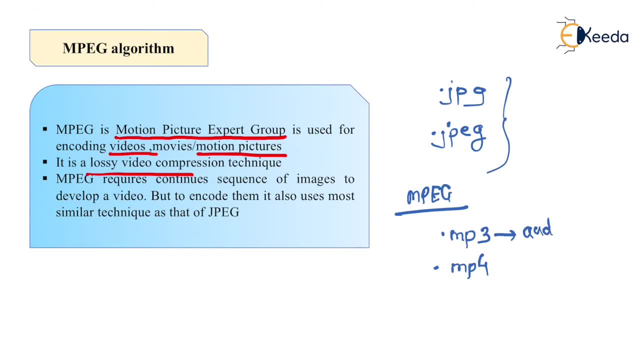 mp3 file is used to store the audio file format, And mp4 file is used to store the video file format. Now, with the help of these two things, we can understand that MPEG technology is related with encoding a sequence of images. 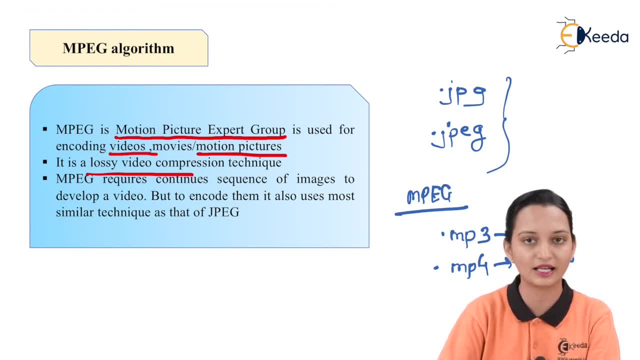 But it can store a file in the audio as well as video format. So the compression technique of MPEG can leads to store all the types of the format of the data With the help of mp3. And with the help of mp4 extension. 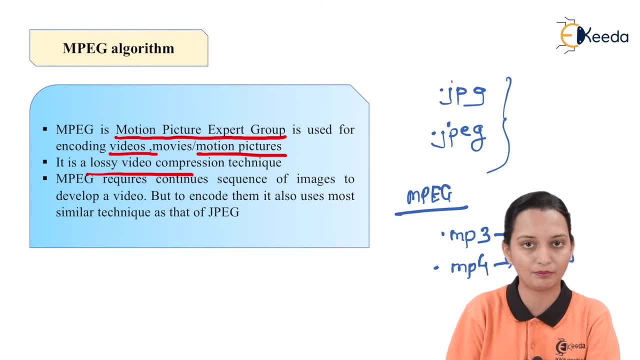 So that there will be some standards of the MPEG which are suitable to store the audio files, to store the video files, And we have to see all the type of standards in detail. Now, as I already told you, the encoding technique of MPEG as well as JPEG are much more similar. 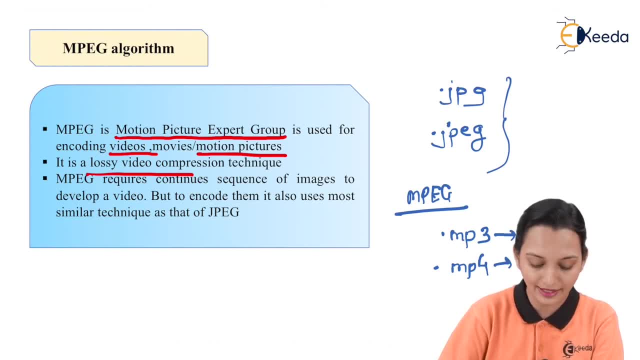 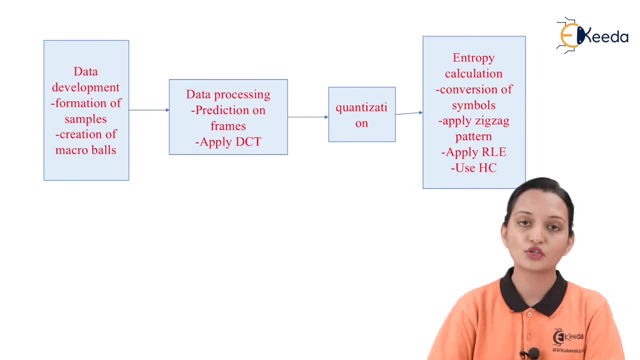 Then we will have a look on the exact encoding technique with the help of MPEG, With the help of MPEG algorithm. So this is nothing but the block diagram of algorithm with the help of MPEG technology. So the first one is data development. 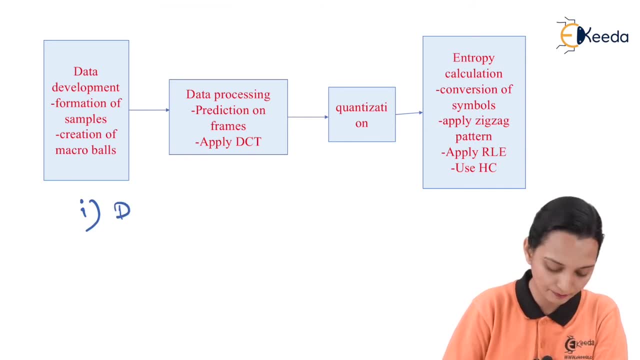 So the first part of MPEG algorithm is data development. Now, in the data development, there will be two main step. The first one is formation of samples And the second one is creation of macro balls. After creating the macro balls, its output, they have to applied for the data processing unit. 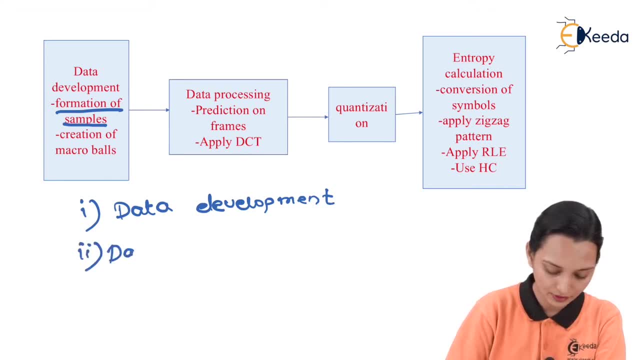 So the next step is nothing but data processing unit. Here again, there are two steps. The first is prediction on the frame And second is apply DCT. Now we all are familiar with this two terms. We have to predict some samples. 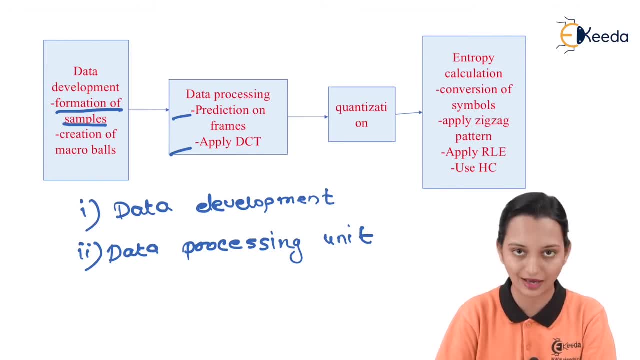 Frames are nothing, but again there will be some sampled values And which on which we have to apply DCT Its output. we have to apply for the quantization. So the next step is nothing but quantization. Quantization means rounding up the data. 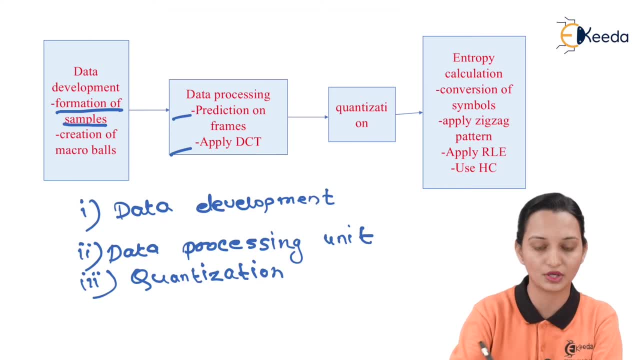 The actual reduction can takes place in this particular step, And the next is entropy calculation. Now why the calculation of entropy is necessary? This is the main question. Entropy is able to gives us the value of efficiency, And efficiency is completely related with our output. 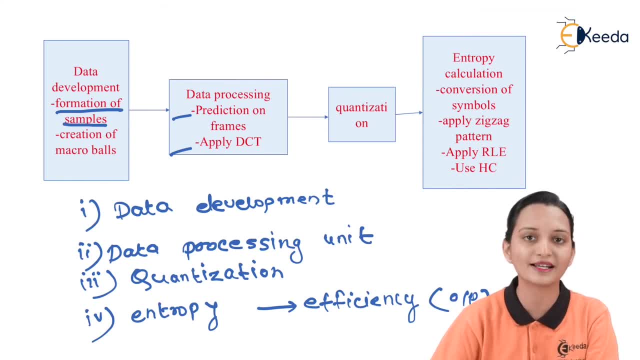 So to achieve the maximum output we require the maximum entropy. So the conclusion of any algorithm or the conclusion of any example is nothing but the value of the entropy. So there is a necessity to calculate this entropy. Again, for the calculation of the entropy in this there are three steps. 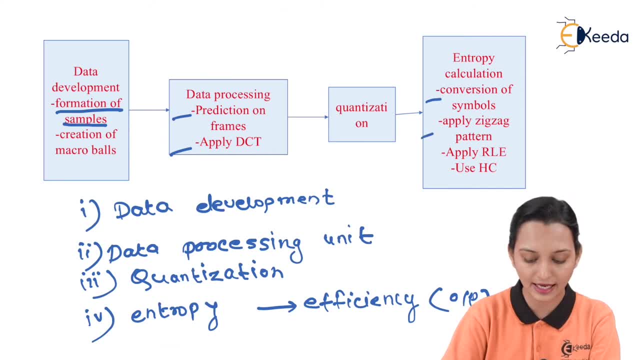 Conversion of symbols: Apply zigzag pattern, Apply RLE And use XC. RLE means run length encoding And XC means Huffman encoding. So we all are running, We all are familiar with this particular block. That means for the entropy calculation. 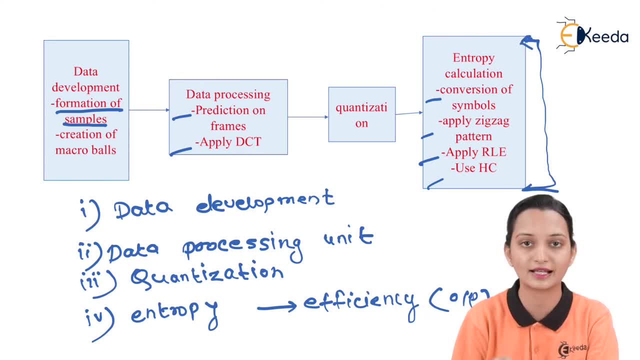 Because this technique is completely similar as that of the JPEG algorithm. Now we have to follow these four process and their sub steps to calculate the MPEG output. So how, on every step exactly, we can calculate the output, and that we have to understand. 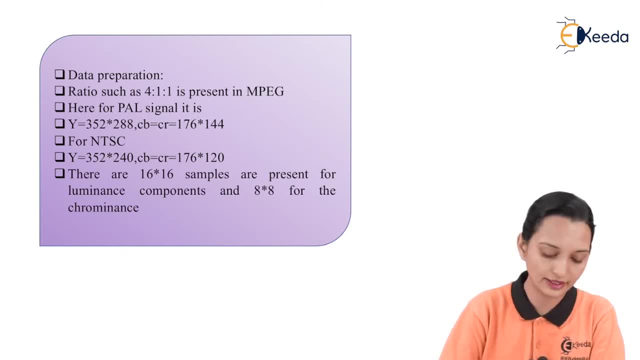 So this is the step number one: Data preparation. In that there are again two steps that we have seen Here. we have to take ratio such as 4 as to 1, as to 1 is present in MPEG. Now, what is this? 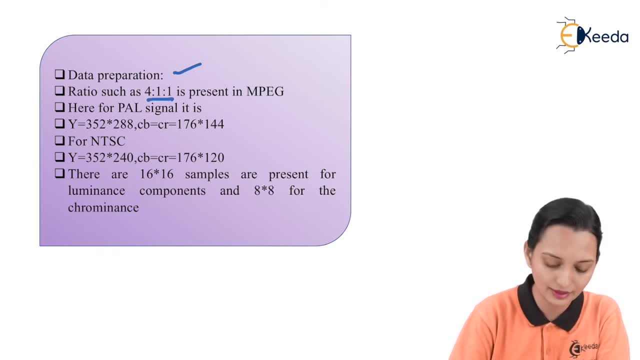 Any image can contains color, Color in the form of RGB That we can convert into the different form, YCBCR. Here Y is nothing but brightness, Brightness of your image or of your video. CB is nothing but blueness in your image. 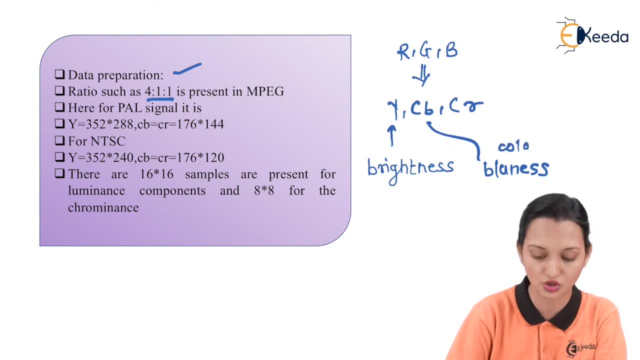 That means the color blueness in your complete image. We are not talking about part of the image. This is nothing but the calculation of our complete image, And CR is nothing but color redness. That means how much percentage of your particular image. 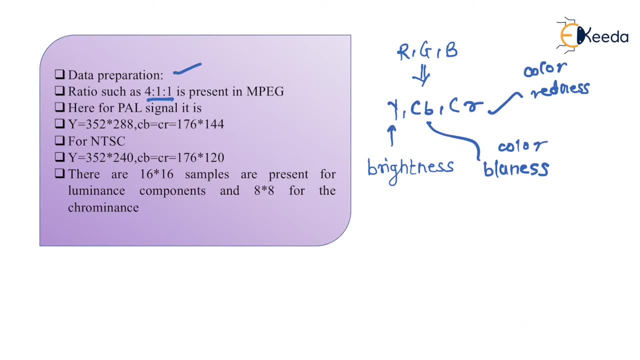 Of your particular input is having the red color. Now, this CBCR are nothing but C1 and C2.. They are known as chrominous signal And Y is nothing but brightness of your image And it is known as luminous part of your image. 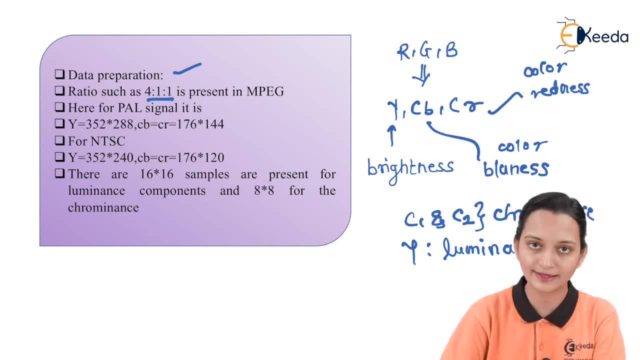 That means the brightness of your image. So Y plus CB plus CR will gives you a complete, developed image. So this is the ratio of this YCBCR. So brightness is present at 4.. As to CB is present at ratio 1.. 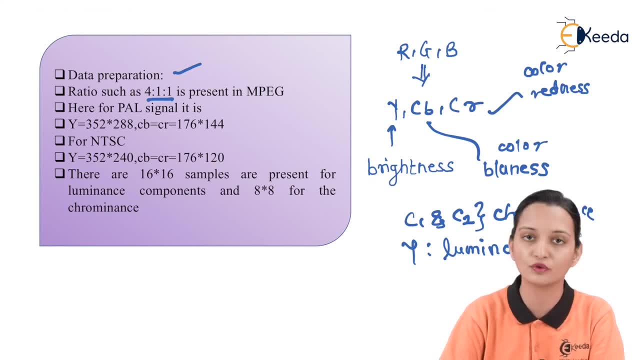 As to again, CR is present at ratio 1.. This is the standard format of the color combination, or YCBCR ratio In your MPEG input. So this is the ratio, Such as 4S21S21 is present in what? 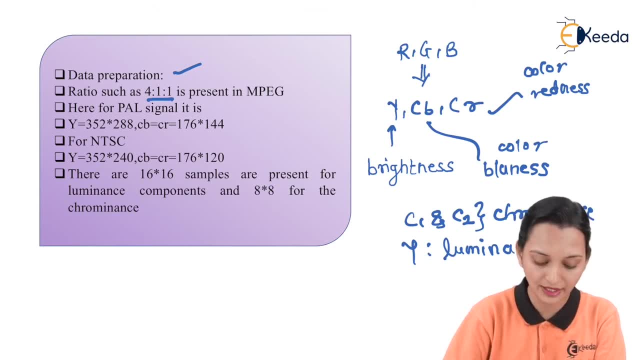 Present in MPEG. Here for PAL signal it is. That means the value of Y, CB and CR. They are 352 into 288.. Now, what is this? Any image contains some brightness, So contains some CB, contains some CR. 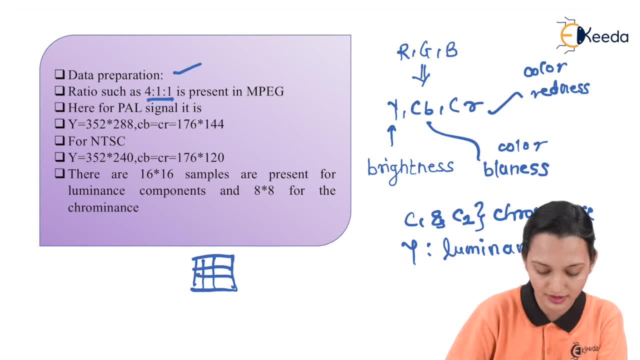 So how we can calculate it? This is nothing but what. Suppose this is a matrix of a image, Given image of X into X or X by X matrix, Then the height and width Of this particular matrix Will give you an idea about. 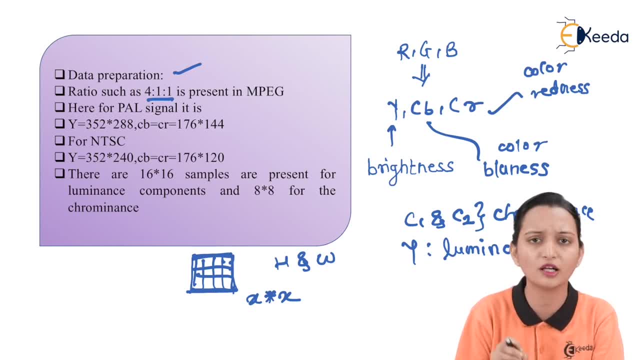 The number of pixels present in the matrix, What it means by number of pixels. Every block is able to represent the pixel. So if I want idea about the number of blocks Or number of pixels in the matrix of an image, I must know the height and width. 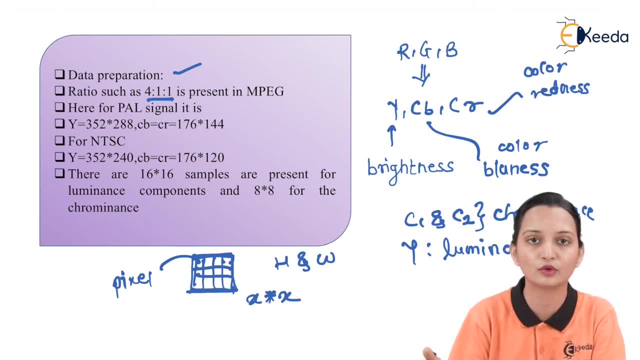 So that I can take the multiplication of them To calculate the pixel or the block Numbers. So suppose our matrix is of 2 by 2. Then height is 2.. Width is 2. So how many blocks will be present in my matrix? 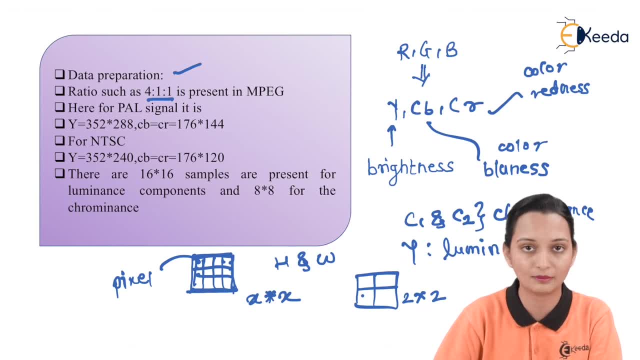 1, 2, 3, 4.. 2 into 2.. How many pixels can be present? Again, the number of blocks, Or every block can contain the different pixel And every pixel can contain the different values. So that is the calculation of the actual pixel. 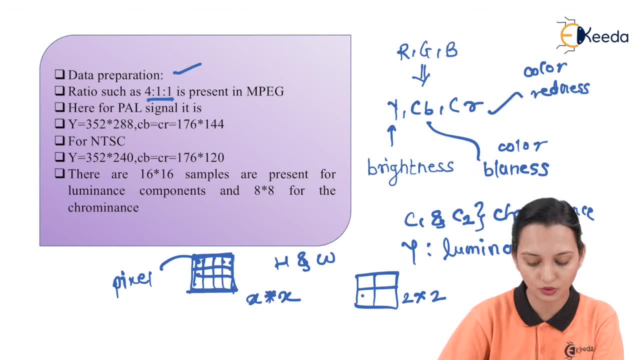 The total value of pixel is a different thing, But the total amount of blocks present in the picture Is nothing but what Height into width of that particular matrix. So Y is nothing but the luminance And its value is 352 into 288.. 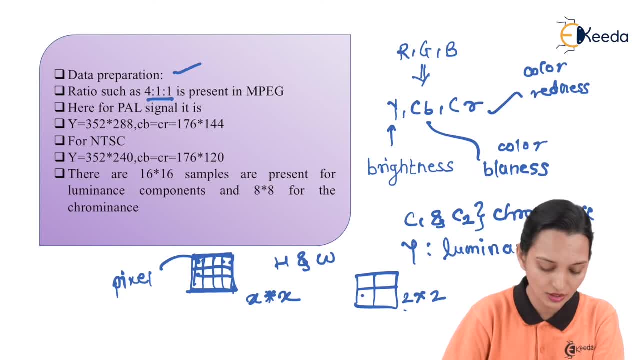 CB and CR. both are having the same proportion. So that is nothing but 176 into 144.. This is the value of CB and CR. Now, this is for PAL signal, Like that. there is other one more signal present, More signal present in the MPEG. 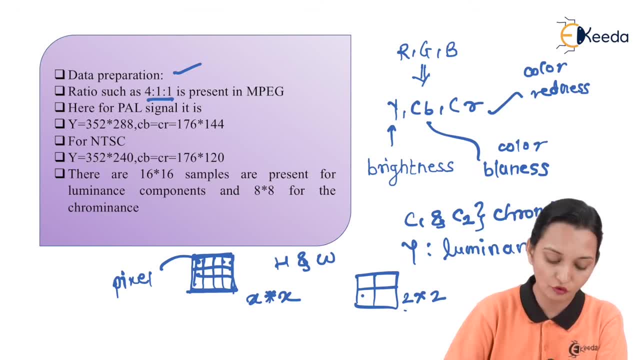 And that is nothing but NTSC. For that particular signal, Again, there are different values. They are nothing but 352.. Height is same, But width: 240 is the width Here. also, height is same For CB and CR: 176 into 120 is the width. 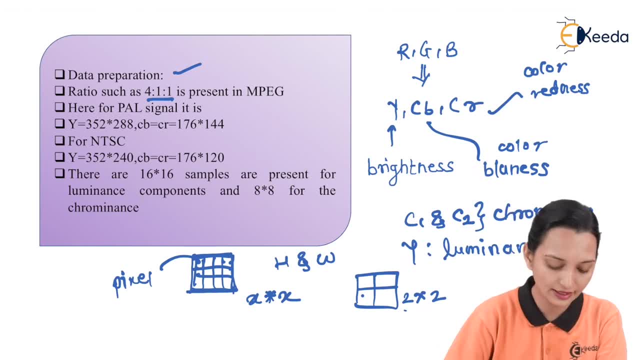 So there is a difference between the width of the image And that will provide such two types of signaling: PAL and NTSC. So depend on a particular application, We can go for any type of a signal. There are 16 into 16 samples present for the luminance component. 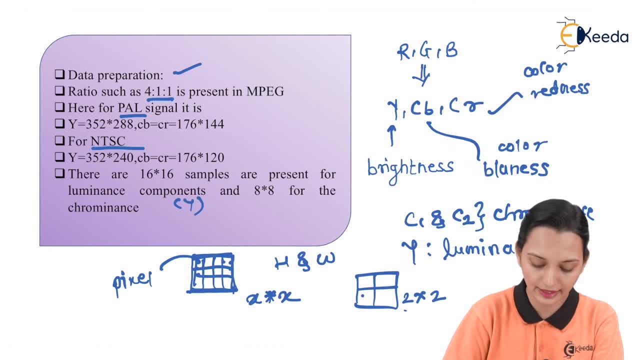 So this is nothing but what Y component And 8 into 8 for the chrominance. So this is nothing but C1 and C2.. And most probably now it is known as what CB and CR, Because we have taken the CB and CR. 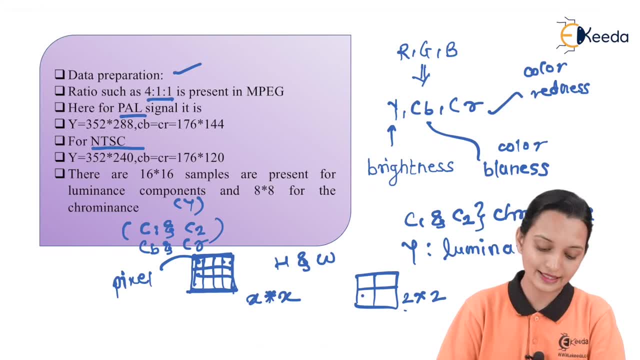 As a C1 and C2.. So this is the second step in the data preparation. The first step is nothing but what Color combination, Their size. So in the data preparation, There is this first step And this is the second step. 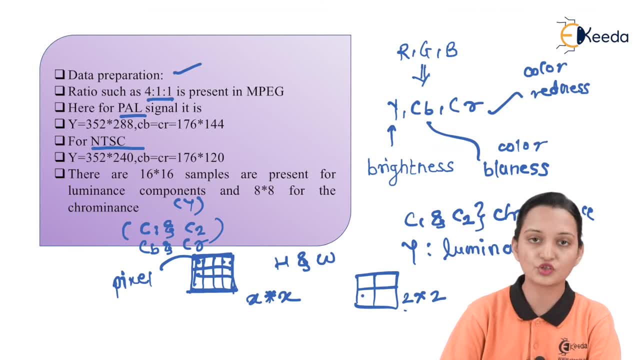 That is nothing but what Selection or the creation of macro balls. So there are 16 into 16 samples are present for the luminance component, That means Y, And 8 into 8 for the chrominance, That is, for C1 and C2.. 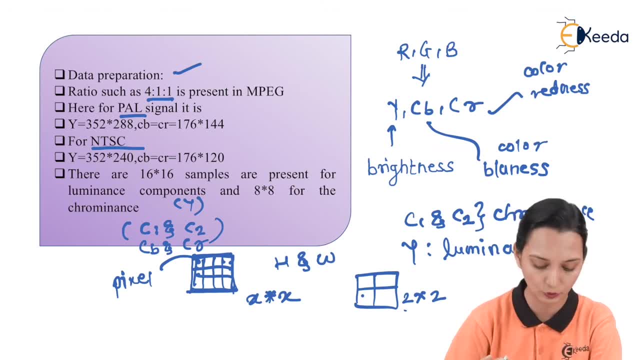 And here CB and CR are going to replace C1 and C2.. So this step is nothing but creation of macro balls, And these are required to calculate the actual output with the help of the MPEG. So creation of samples is the step number 1.. 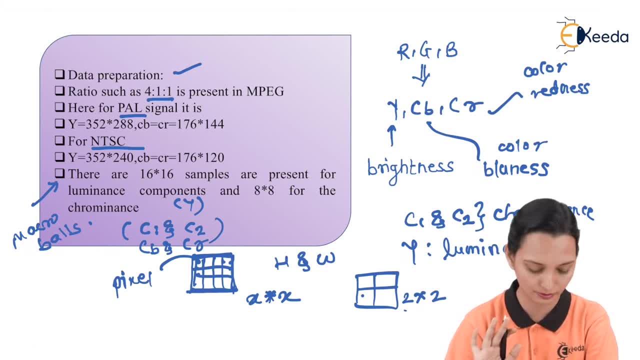 Creation of macro balls with the help of that sample is the step number 2.. So what actually happened? 16 into 16 samples of luminance And 8 by 8 samples of chrominance are present in a pixel, For example. if I am going to draw an image, 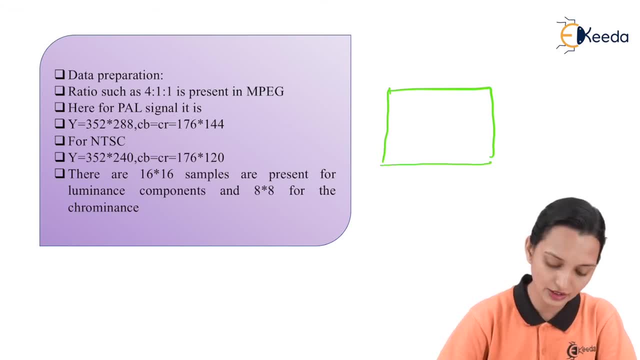 Image size, having 16 into 16 samples. So how many rows and columns will be there? Hopefully you can understand. These are the 16s, And the rows will be also 16s, And hence this can be known as, or can be treated as, 16 by 16.. 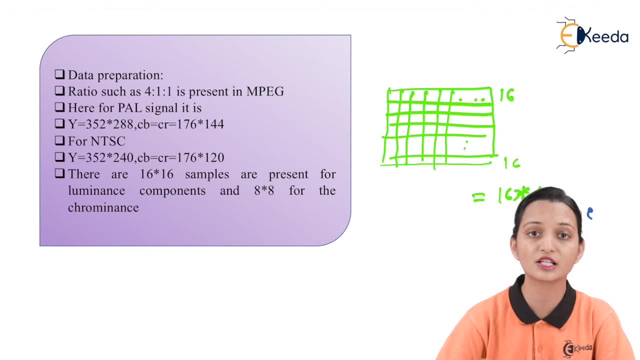 So this is nothing but what Luminance? Luminance means brightness, So obviously if I want to observe the image, I require the brightness. So to hold complete image, whatever it will be, For example, I want to display a number like 8.. 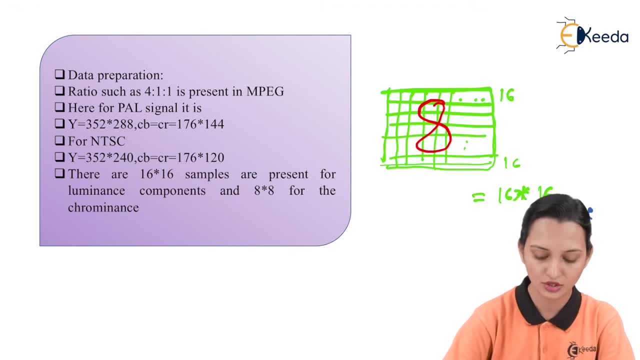 So this is the actual image on which I have to focus. So this is the image part on which I have to focus, And this is the image part which is nothing but can be considered as a background of the image. So, simply, MPEG will do what. 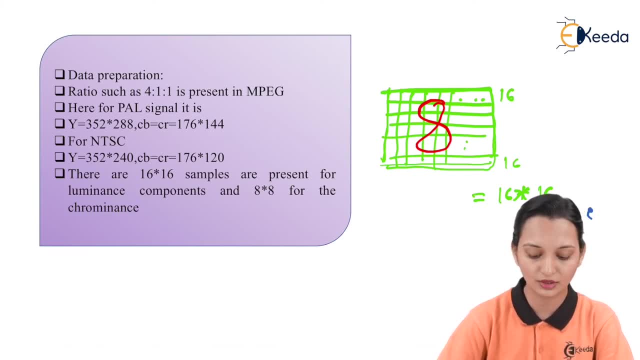 MPEG will try to do some algorithm or do some coding on the focused part And the unwanted part that can get removed And which is nothing but what Actual data? Yes, it is present in our particular image. This background is present for our particular image. 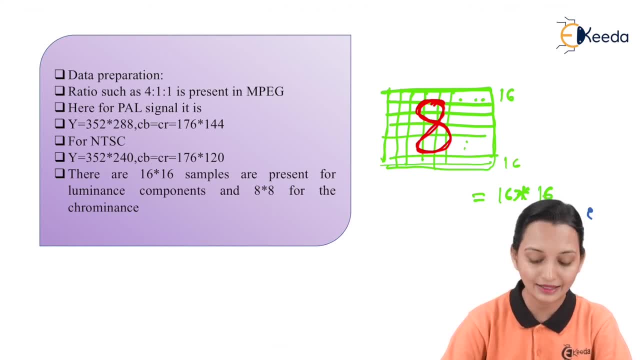 But it is an unwanted part, So that part can get lost during the transmission And at the output we can get the focused part- Most probably focused part- instead of the unwanted part And in this way it can do the lossy compression. 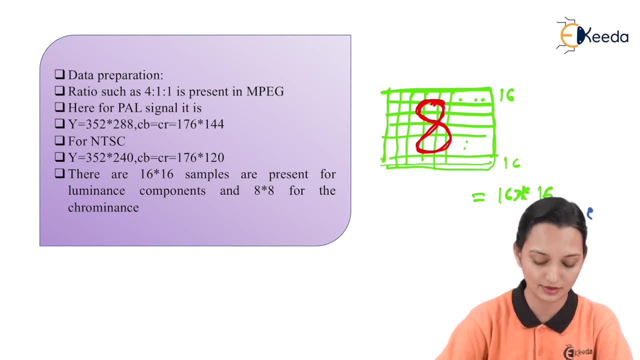 Now we are here, We required to select the samples which are having the luminance and chrominess. So luminance is nothing but brightness. We required the brightness to our image So that can be provided to a complete image That is 16 by 16.. 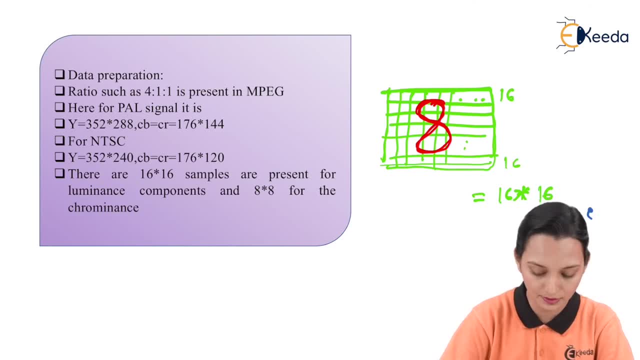 But what about chrominess? I already told you Chrominance is present with the help of CB and CR. That means blueness of image And redness of image. So this is nothing but the blueness of a image can be present in few part of the image. 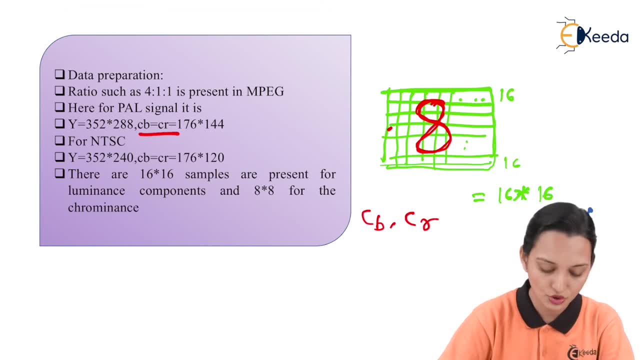 It cannot be present in a complete part of the image. So what are the ratio or the proportional where it is present? 8 into 8.. That means not a complete image can be made up of only red color. It cannot possible that it will be made up of only blue color. 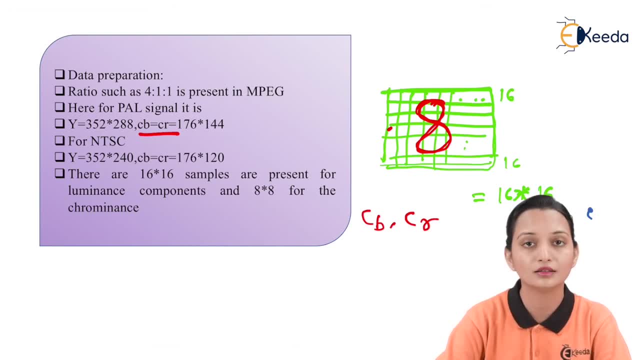 So the few part instead of 16 by 16.. The 8 by 8 samples are made up of CB. The 8 by 8 samples are contains CR. So this is nothing but what A complete image can be developed with the help of Y, CB and CR. 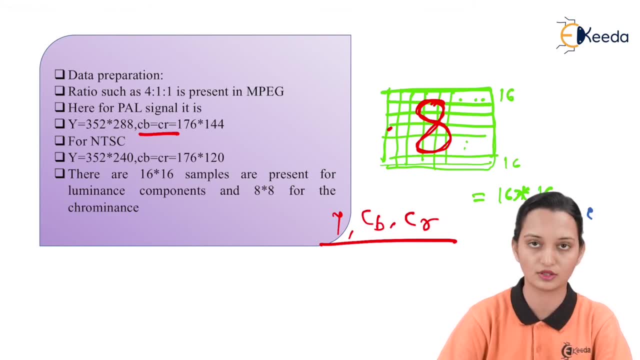 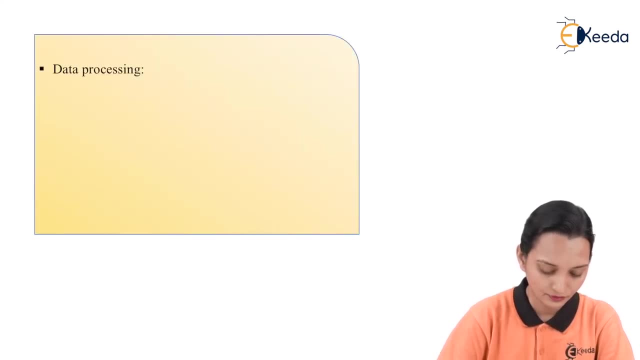 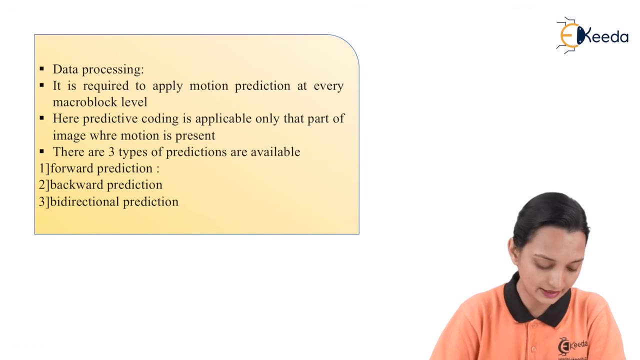 So this is the second step where we can create the macro balls. This step is known as the creation of macro balls, So, actual, the step number second is data processing, Once we are getting the samples and macro balls, with the help of the step number one. 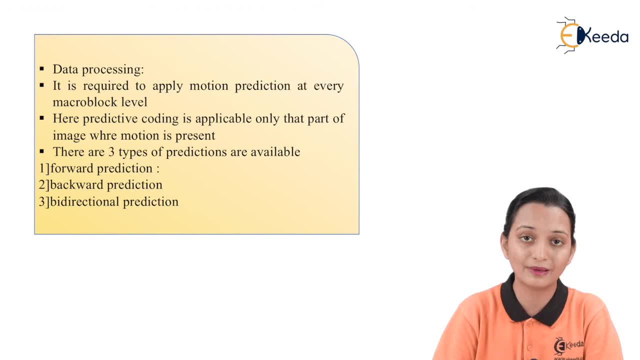 Which is known as the data preparation. We can move by taking the output from that step towards the data processing, Which is the actual second step of your MPEG algorithm. Now, what happen in data processing? It requires to apply the motion prediction at every macro ball level. 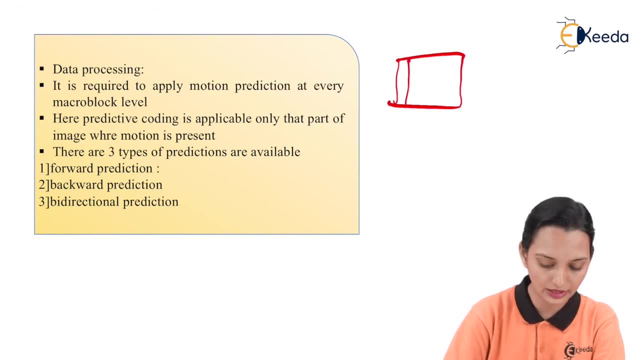 Now we are here, We try to develop a image. An image and that image contain a particular number, For example. this is our the output getting from the step number one. Now it is required to apply the motion prediction at every macro balls level. 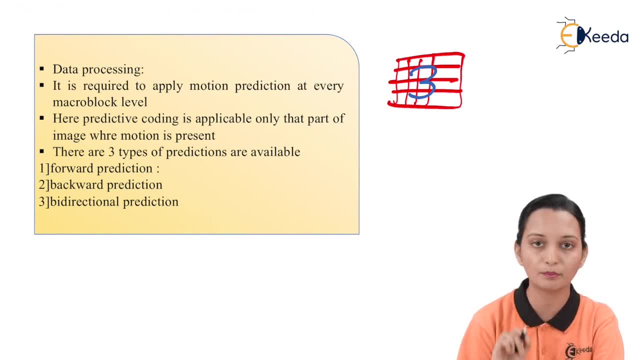 MPEG will do encoding only in the part of a motion, Only in the part, Only in the part Which is in motion, So that we can get the actual output in terms of the video compression, The part which is stable. We can treat it as image. 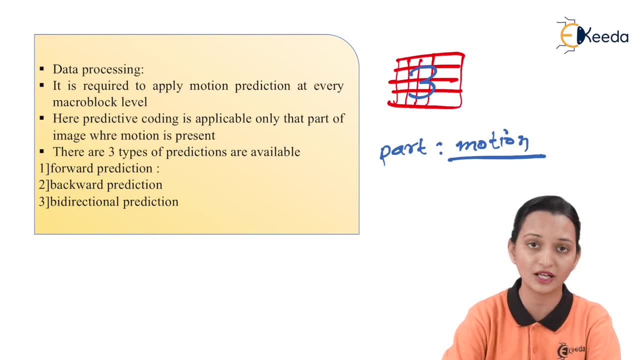 And we can encode that particular image with the help of JPEG also. Then what is the use of MPEG? MPEG is used to encode the video, Is used to encode a sequence of images, That means the motion pictures, So that a part which is in the motion form. 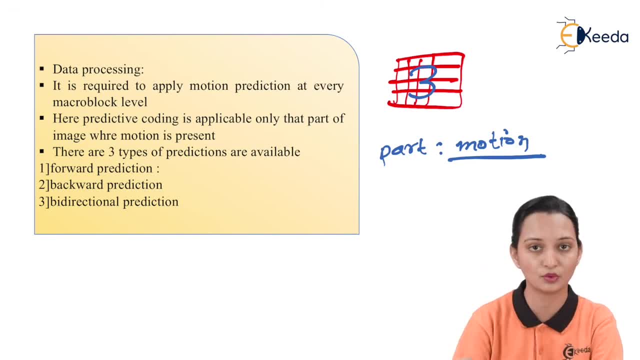 That can be encoded, Or on that part only, we have to focus for the encoding. So we have to predict, Because each and every macro ball is not giving us the motion value of a picture. So we have to predict a motion, So that we can apply a motion prediction at every macro ball level. 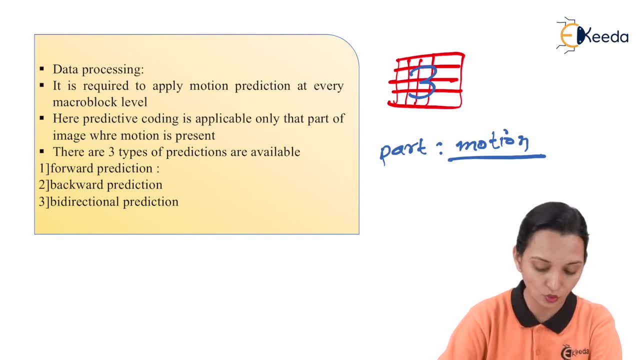 Here the predictive coding is applicable only that part of image where motion is present, And this is very important point, That on which particular point we are going to focus in our image. So there are three types of predictions available. The first one is forward prediction. 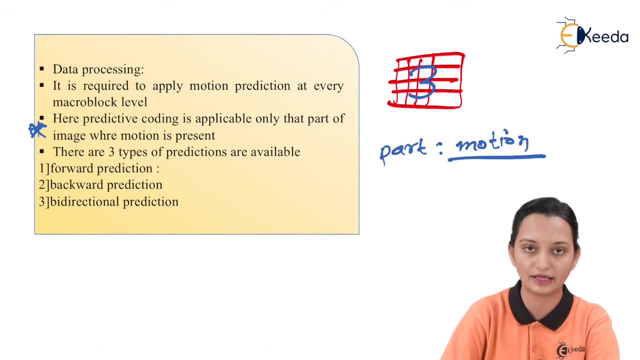 Second one is backward prediction. Third one is bidirectional prediction. Forward prediction can apply with the help of the previous image Or the past images. Backward prediction can be applied with the help of The future or the next Next frames, And bidirectional prediction is nothing but the combination of both the things. 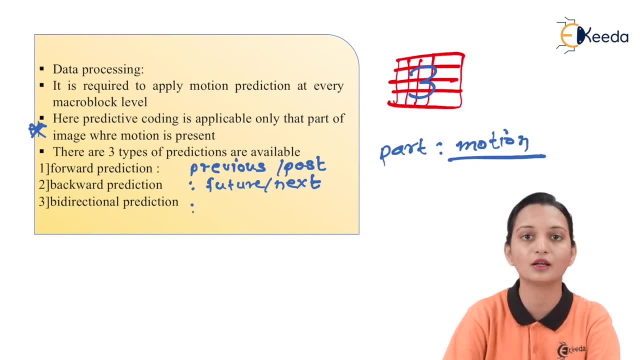 And we have to apply the bidirectional prediction as per the requirement of application. So the forward prediction and backward prediction, These are depend on the frames. So first we have to understand what it means by frames. Every image is nothing but The combination of different frames. 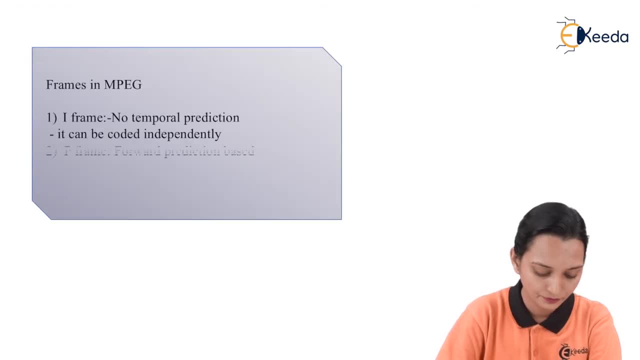 So We will try to understand the frames in MPEG. So first is the I-frame. I-frame contains no temporal prediction. That means, whatever the output which you are getting at the present step, Take that output and try to encode the data. It can be coded independently. 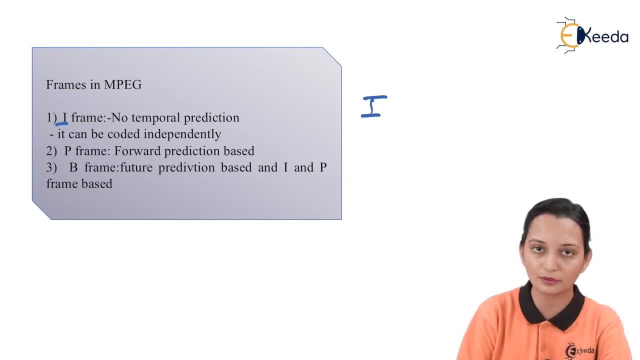 Yes, Why? Because it is not depend on the backward prediction. That means you are the previous frames. It is also not depend on your future frames And also it does not contain any prediction. So the actual value is nothing but the output coming from the I-frames. 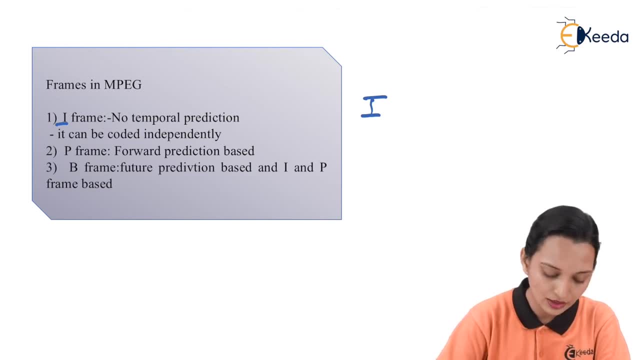 So it can be coded independently. Then next one is nothing but T-frame. It contains the forward prediction based scheme. That means what Forward prediction means what That value is depend on the value coming from the back frames or the previous frames. And the next one is B-frame. 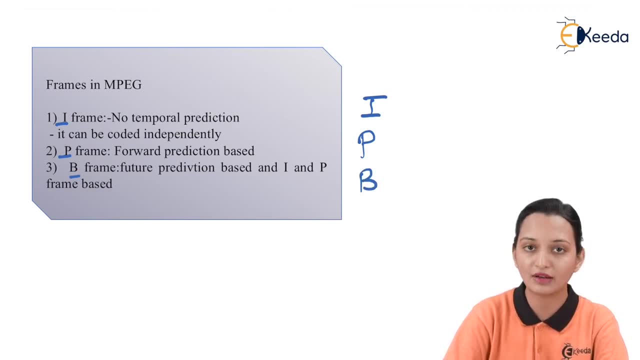 Future predictive based. That means what The value is depend on the future frames prediction And I and B-frame based Indirectly what Both the frames enter. output: Yes, It will contains the output depends on I as well as P-frame. 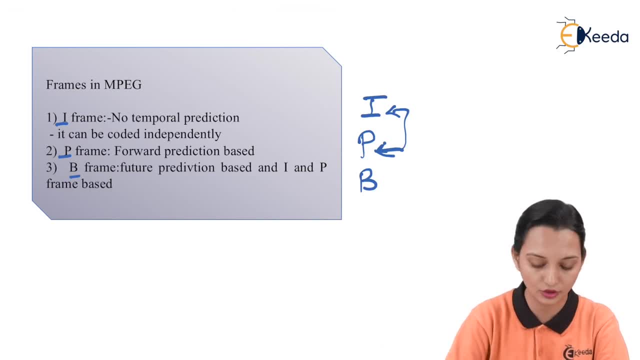 So, first of all, the I-frame current value, So independently coded P-frame. it based on the forward prediction That means the previous value depend on, And B is nothing but the combination of I and P-frame. So, with the help of I, P, B. 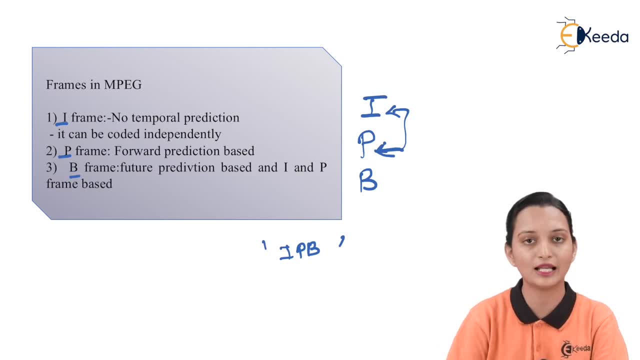 This is nothing but the frames in the MPEG. With the help of the values getting from this particular frames, We have to encode or we have to predict, actually the motion prediction So that we can encode a particular video. So here is algorithm, or this output we can use where 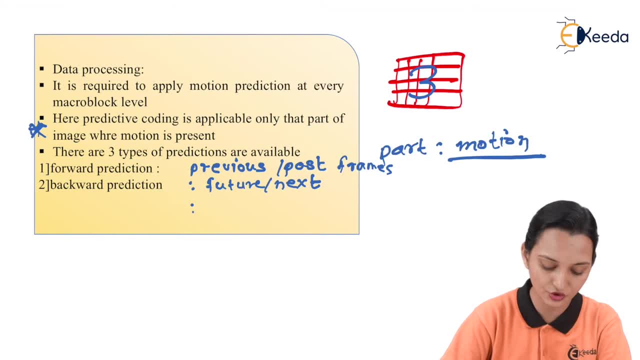 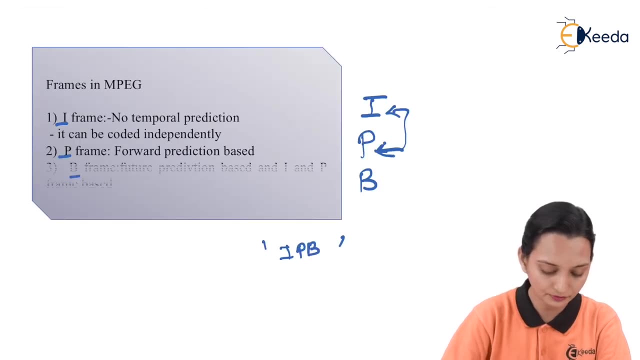 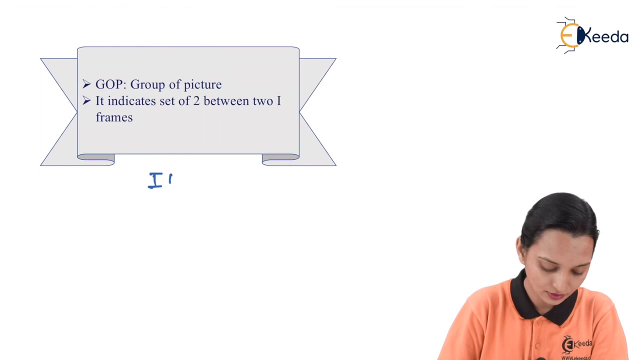 We can use that particular output in forward prediction, in backward prediction and in bidirectional prediction. So with the help of these three frames we can do the motion prediction. That means the data processing. Now the next part is once we have the idea about I P, B frames present in a particular input. 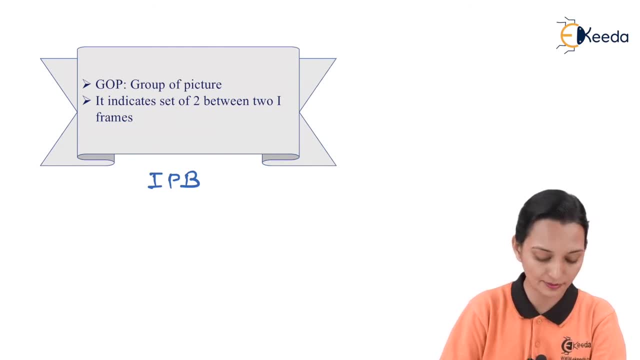 We can calculate the GOP- Now what it means- by GOP. Group of pictures. It indicates set of two between two I-frames. Now what it means exactly. For example, If your particular input is nothing but the development of I, P, P, P. 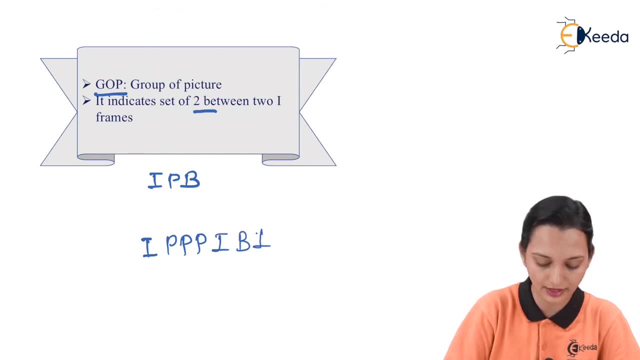 Again I, again B, again I, again P, again I, then I, I. This is nothing but, for example, development of your image, Or we can say multiple image, Single image, Or indirectly, the input for your MPEG. Then this is nothing but the frame structure. 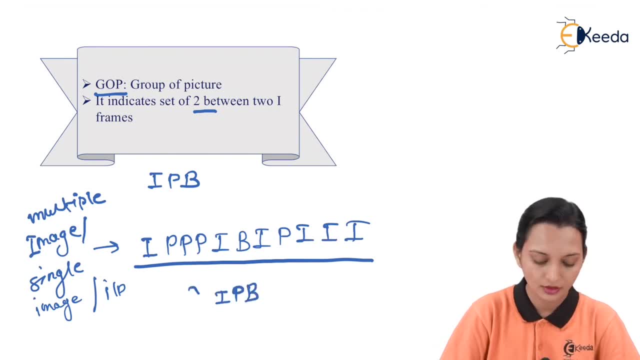 That is a combination of I, P, B. Then how we can calculate the GOP. It indicates the set of two between what Between two I-frames. So, from this I to the next I, What is this Set of two I? 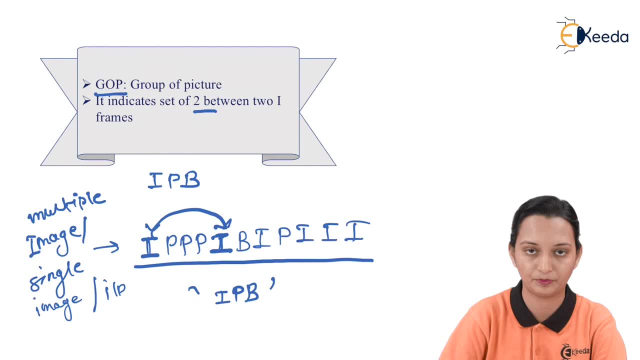 And in between that, how many frames are there? Three P After that. again, this is the new I. This is the next I, So set of this two I And what it in between. B is present, B frame is present, So B frame is nothing but what. 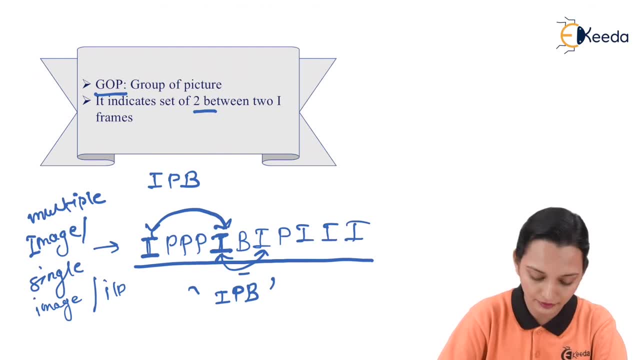 Group of frame In between this two, I Again, in between this two. I What is present, The different P-frame. So P-frame is nothing but the group of frame Which is present in between two. I After that, in between this two. I. 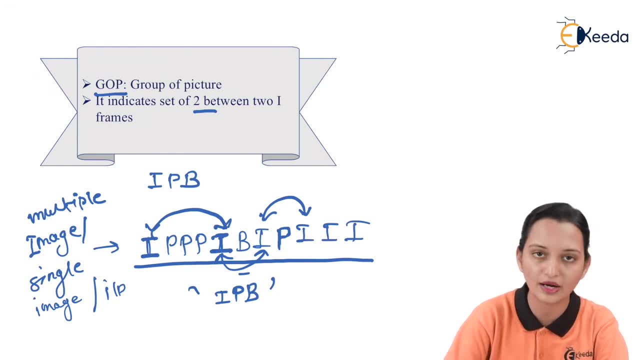 II is nothing, but what Between two I So II. This can be a single group, This can be a single group, Or this can be a single group. So in between two: I, Whenever something is present, Or the group of I. 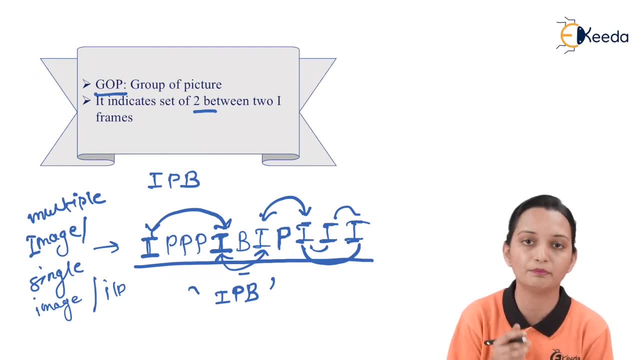 Or the group of any frame of I, B or P. That is nothing but known as the GOP. And such kind of GOP Are much more useful for the motion prediction. So can So that we can predict a motion of a picture. 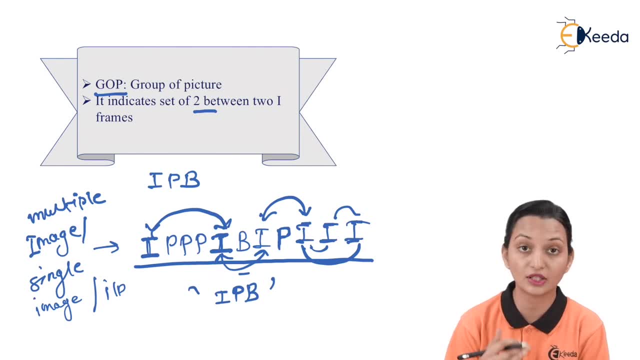 So the development of frame is necessary So that we can calculate the GOP And then we can go for the forward prediction, Backward prediction By direction prediction To calculate the motion prediction. Motion prediction is useful for the Selection of a motion part. 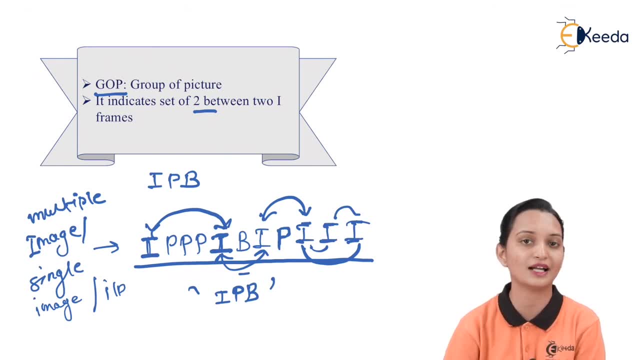 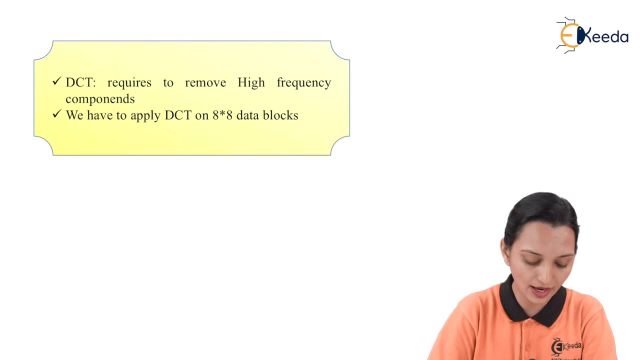 In a particular input So that we can encode that part. The next step is We have to apply DCT On what On the required To remove the high frequency component? Why to apply the DCT For removing high frequency component? 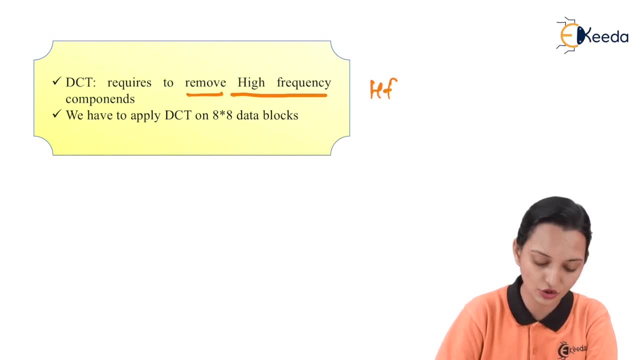 HF component. We have to apply DCT on what On eight into eight blocks, So eight by eight blocks, Which are able to give us some coefficients. How many coefficients? they are able to give us? Sixty four coefficient. So on that particular coefficient, 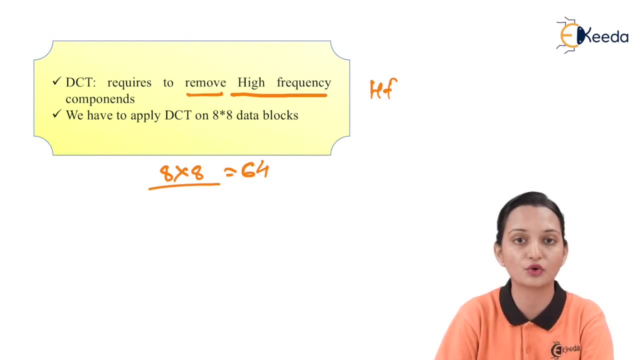 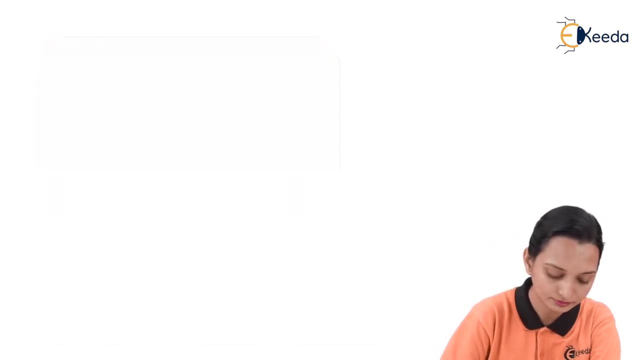 We require to apply the DCT To remove the high frequency coefficient. That means indirectly, We have to focus on the lower frequency coefficient. And next one is quantization. Apply this process on a frequency domain, coefficient. Now, quantization is nothing but for rounding up, 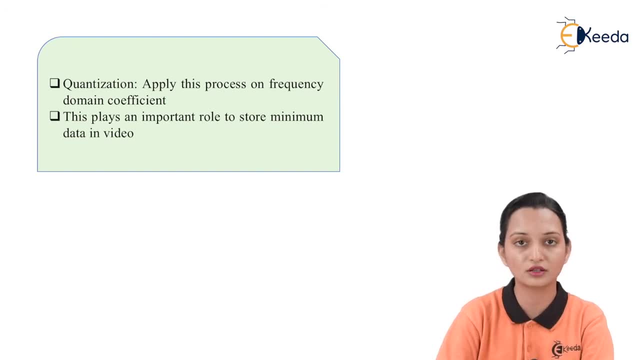 The sampled value To reduce the data In your input. Now we have to apply this particular process To reduce a data, But with the help of what Or on which We have to do this process? On frequency domain coefficient. Now, these are nothing but what. 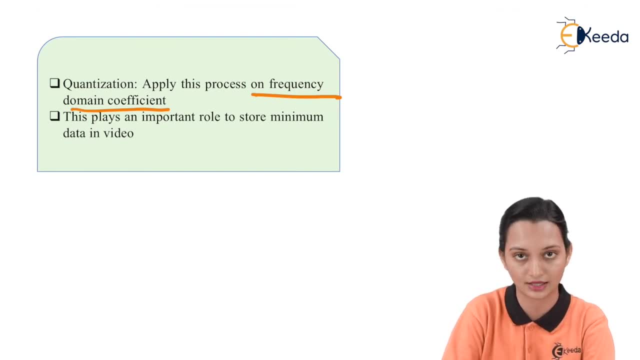 Value Sample, the value Which we can get from the matrices. And to the quantization, Who will provide the value? DCT algorithm output Are nothing but the input For the quantization process. So we have to apply the process. 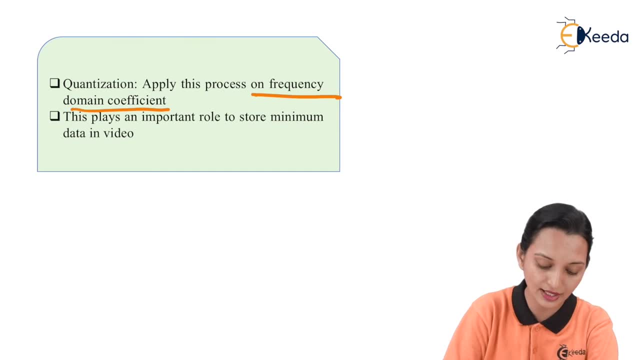 On the frequency domain coefficient only. This play an important role To store the minimum data in a video. Minimum data storing means what? Already we try to remove the high frequency component With the help of DCT, So that what we can save? 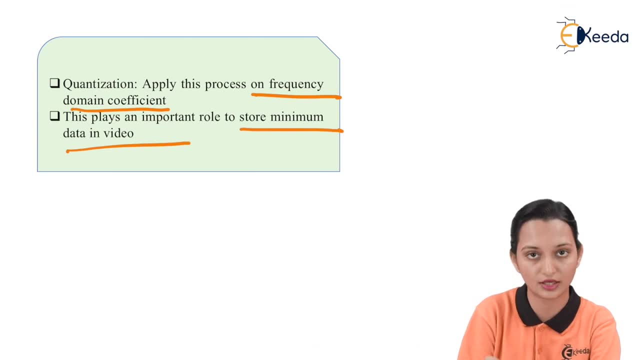 We can save the data space To store a video. After that we try to do the process of quantization, Which is nothing but what? The actual reduction of a process In which we can Apply this process On a frequency domain coefficient. 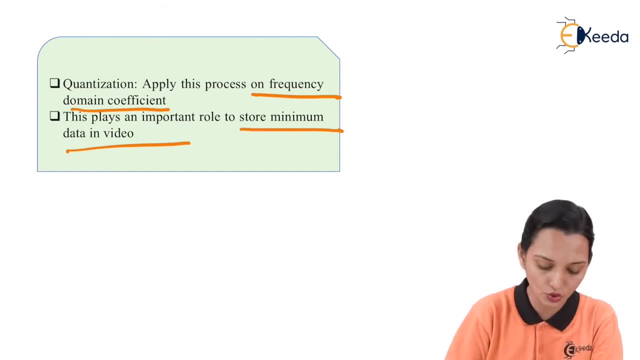 Again, we try to focus on the lower frequency So that, with the help of these two process, We can store a minimum data. That means here, actually, we can Reduct the data. So it plays an important role. For what? For storing the minimum data. 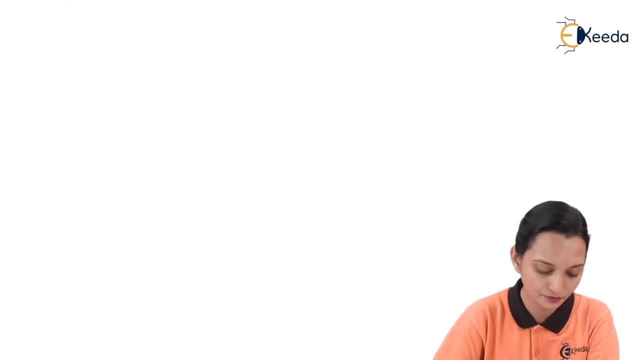 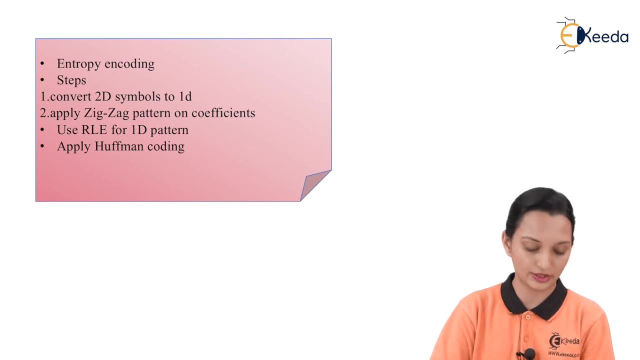 In a particular video. Now the shape number four For the MPEG algorithm. That is nothing but what Entropy coding. I have already told you Why the entropy is necessary To calculate the efficiency of your output, And which will be the aim from any algorithm. 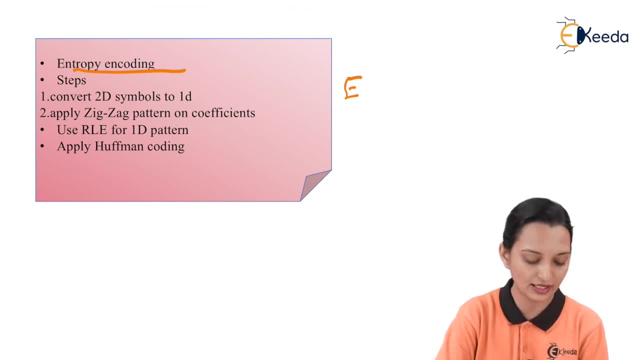 Now to find out the entropy. There are again few steps. First is Convert two dimensional symbols Into one dimensional symbols, So indirectly, conversion of two by two matrices Into one by one matrices. Then second is This exact pattern on the coefficient. 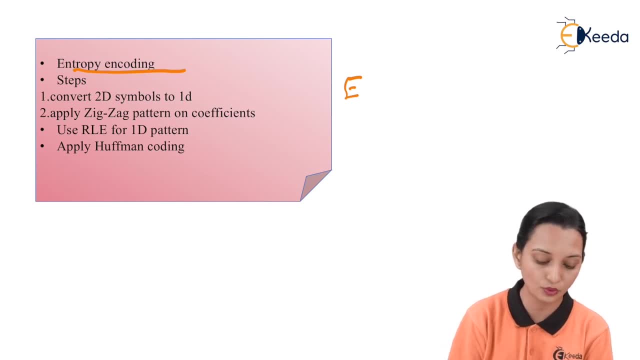 Calculation of the entropy We have to do in this particular step With the help of selection of position, of coefficient, And how can we select the position At which particular step, Which position value I have to use From the given matrices, For example: 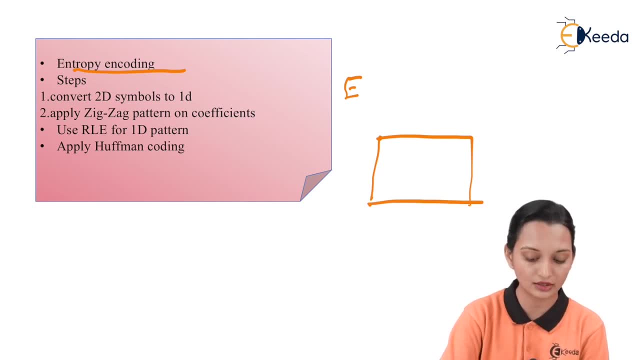 We have already discussed, We can develop an micro balls Having the sixteen by sixteen Value of a matrix. So, for example, This is nothing but A given matrices. Then we have to apply a zigzag pattern. So how can we apply the zigzag pattern? 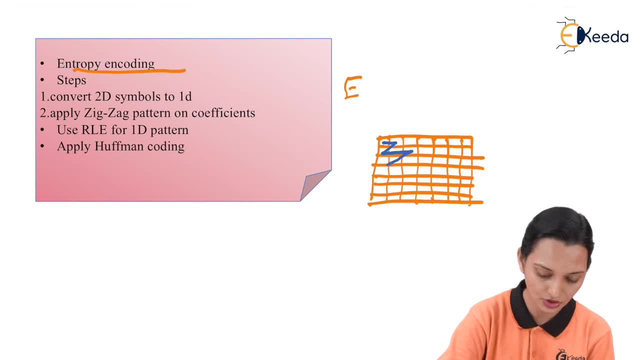 This is nothing, but what Start from this end here. Start from this end here. So like that, we have to go And we have to use the zigzag pattern For the selection of the coefficient In this process. you can understand We try to remove. 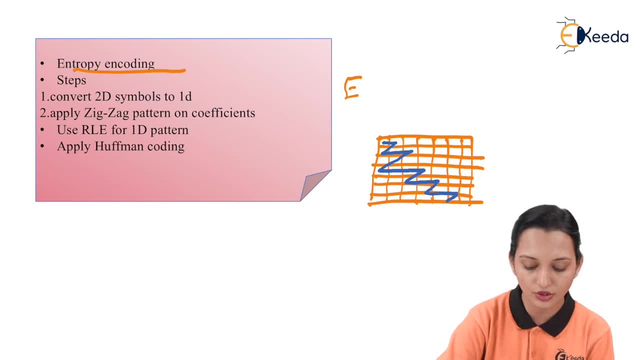 The unwanted data. That means what? We are not going to use, Such kind of samples Or the pixels. Now, the zigzag pattern. We all know This is nothing but what Zigzag pattern, But We can apply the zigzag pattern. 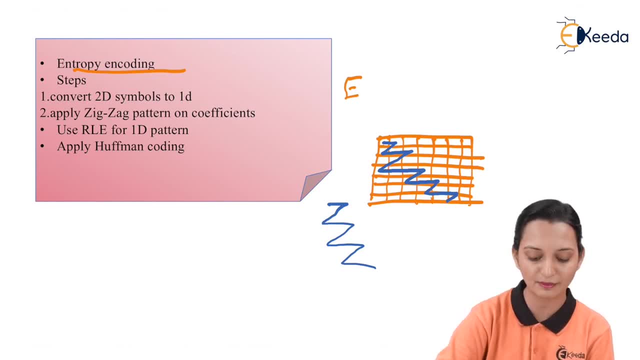 By observing the matrices. Not necessary that Always my matrix will be Like this. That means the size of the matrix can vary When your input will get vary, So that that pattern Where we can apply, Or the pattern of the focused 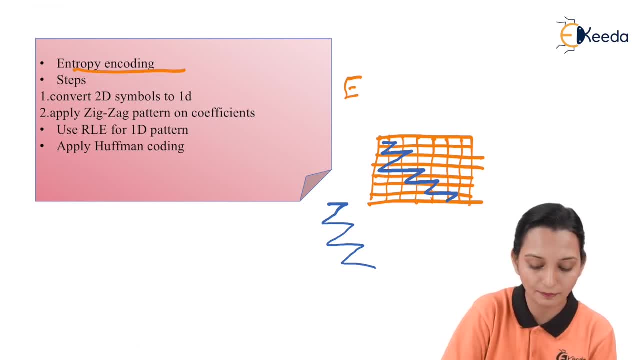 Image can be different. But how to Apply the pattern To select the coefficient? That is nothing but what Zigzag pattern. And it is Fixed Now. the next one is Use of RLE For 1D pattern. 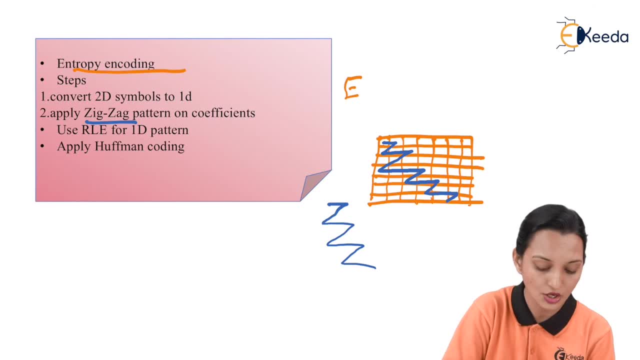 1D pattern means One dimensional pattern. You are getting some output. Now what it means By RLE: 0, 0, 0, 0.. 1, 1, 1.. Now how many bits are there? Total: 7 bits. 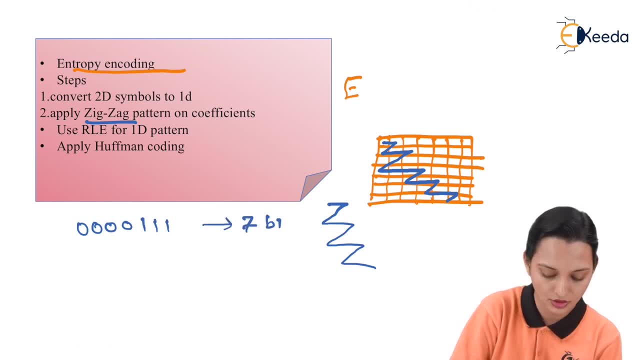 So run length encoding Will give me what: 0, 1, 2, 3, 4. 4 times. Then: 1. How many times 1, 2, 3. 3 times 1, 2, 3.. 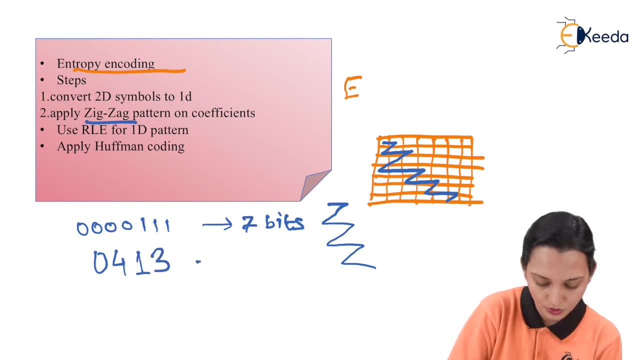 4 times 1, 2, 3. 4 times. So RLE Will gives me The output In the compressed Format. It will never Lose the Actual data. It will try To reduce the size. 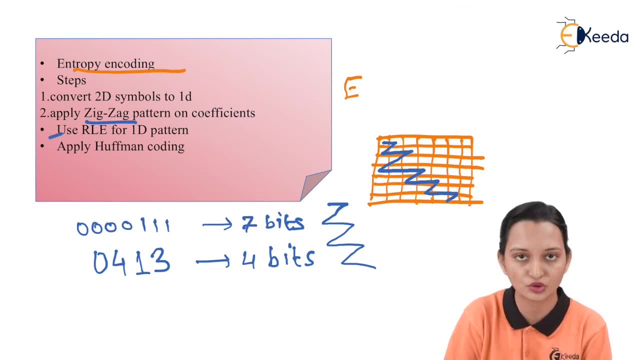 Of the data. So use of RLE Will play Very important Role For the process Of quantization. Now, 0, 4, 1, 3. That means What? 4 times 0 comes 4 times. 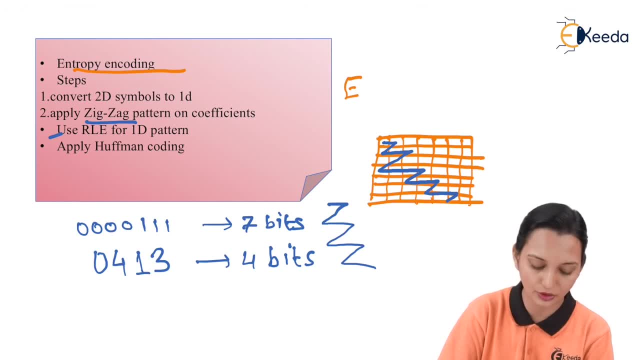 1 comes Or appears 3 times. So at the part Of the decoding I am getting The output Of the Algorithm. Then last Step is nothing But apply Hopman coding. We all know That calculation. 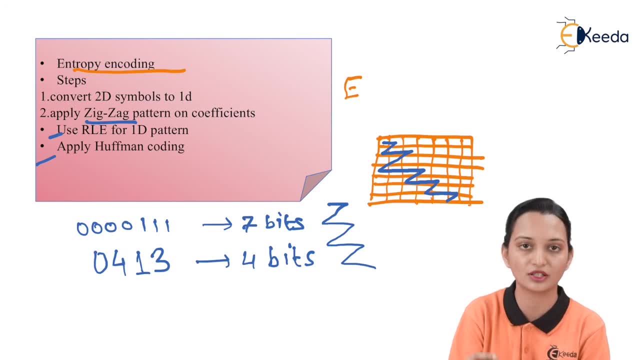 Of entropy Is possible With the help Of some Lossless Algorithm Techniques. Actually, It can be Possible With the help Of lossy Algorithm Also, But already The entropy Value We required. 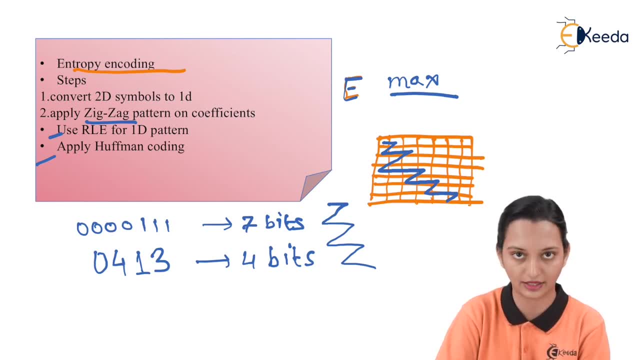 What maximum? Why Is possible Using The lossless Technique? This is The simple Thing Why We are Going For the Alien Hopman Coding: Because These Are Nothing But. 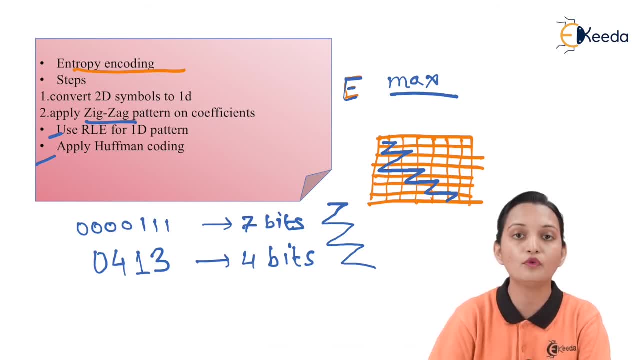 What Lossless Technique? Lossless Means The input Data. After Encoding, You Go Forward The lossless Technology And That Are Nothing But What RLE And Hopman 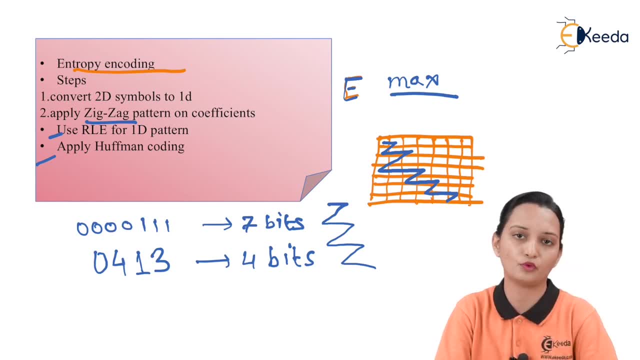 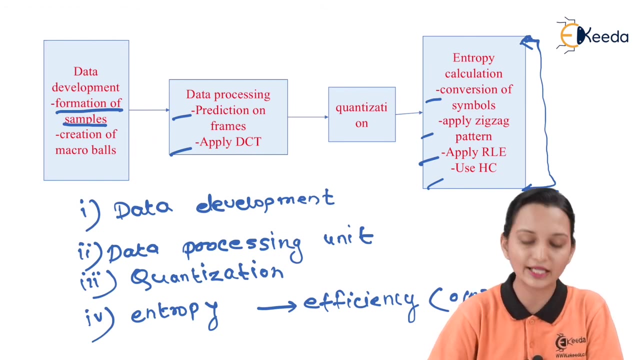 Coding And Hence At The End Of Your MPEG Algorithm, Also Like The JPEG, We Have Made The First Shape Of Data Development. In Which Formation 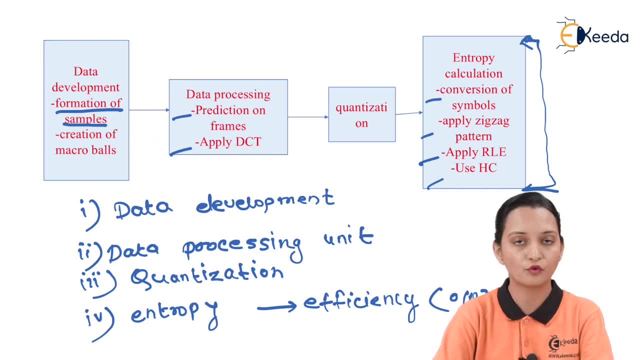 Of Samples, Creation Of Macro Balls, That Means What Y, C, B, C, R And Its Ratio And Creation, B, P, And Then, After Predicting,